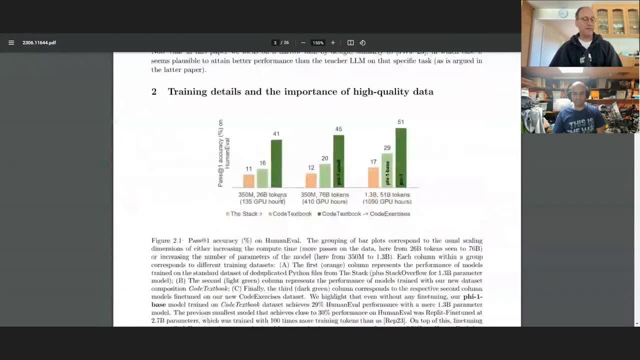 A third thing is, they're seeing more effective results from a much smaller training set, including synthetic data. So I think most people in machine learning look at the training sets they have and the amount of training time they have. 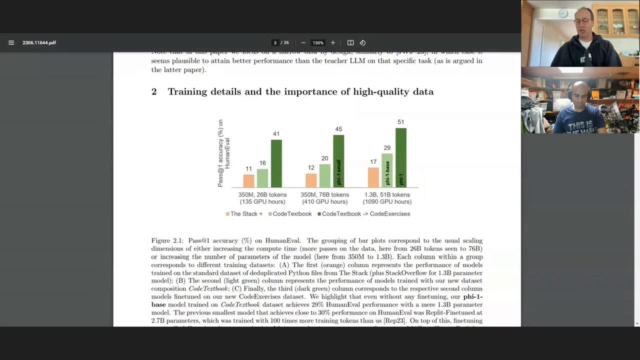 And they say, this is not how a person learns. You're throwing just a massive amount of data at the system. 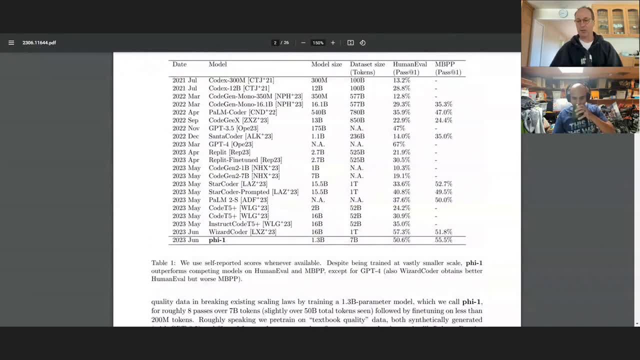 And it's learning usually pretty slowly and then eventually with diminishing returns until you say, okay, I've trained it enough. But a person can often learn something from just a handful of examples, which is a huge contrast to how we train these systems. 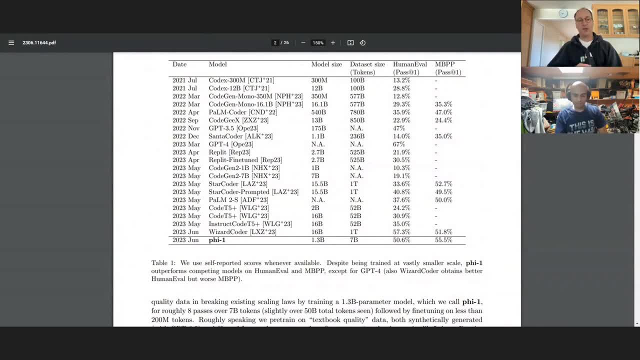 So I think what you're seeing is people realize they're having to train with way too much data for way too long. And they think that there's huge improvements to be gotten from smaller training sets or alternative methods of training. Exactly. 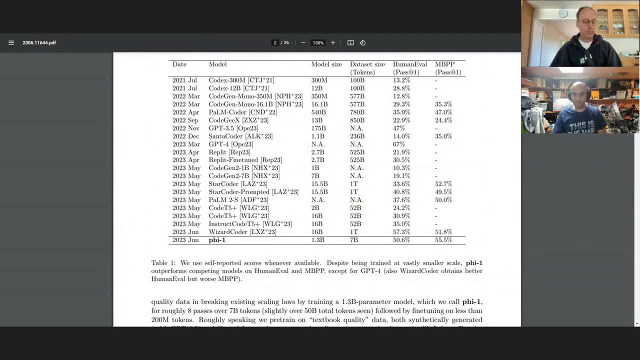 Training sets that have been manicured and are in good shape. Right now, the current debate is Twitter CEO, Red CEO are like, hey, OpenAI was trained on using our data. 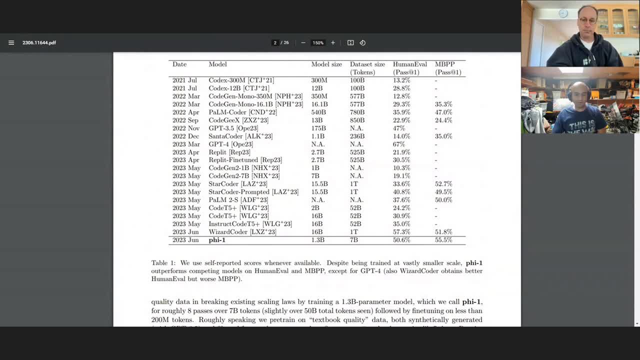 And now we want to start charging AI models for all of this. Based upon this paper, it turns out that, from my understanding, that we... 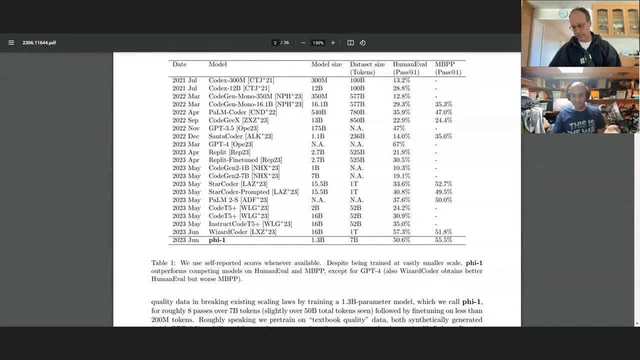 would prefer to train models on structured information, pristine data sets that are near textbook-like quality. So meaning question, answer, question, answer, and no random gobbledygook from crazy Steve about QAnon in the middle, like in Twitter. 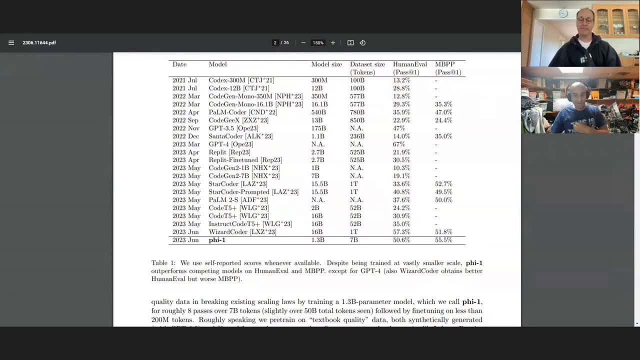 So I think with this, my implication for this paper was, hey, yo, time out. All that stuff on Twitter and Reddit and all the gobbledygook on the internet is slowly losing value in regards to training foundational models. Is that a fair take? I think that's a fair take. 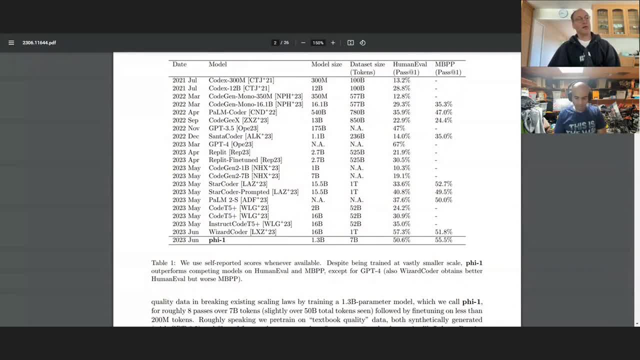 I think that's fair. Curating the kind of training set that you're using, and then also using the training set maybe in a smarter way. 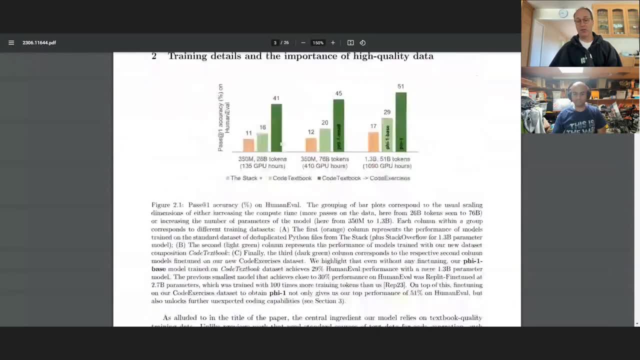 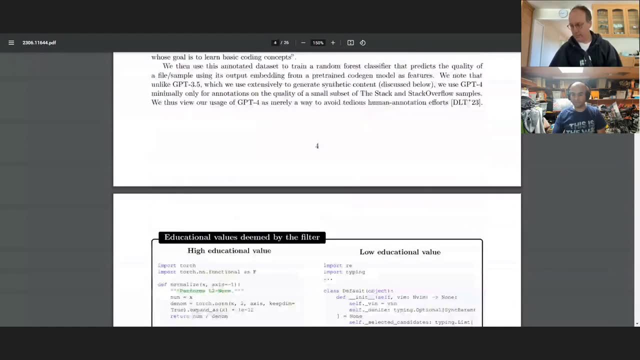 And again, on a much smaller model that potentially could be run locally. I like in this paper also that they're using GPT 3.5 to create questions and answers, and then GPT-4 to review it. 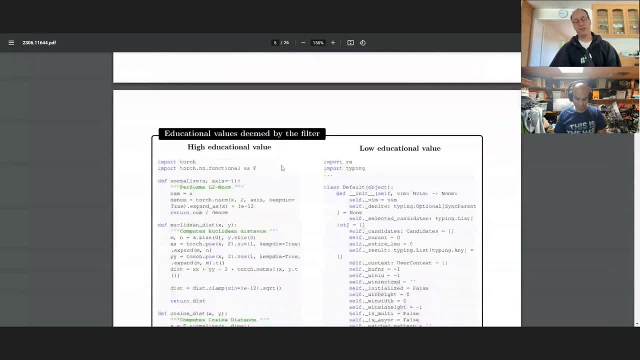 Maybe you can talk a little bit about that. Yeah, we talked about this before with synthetic data. It's interesting because a lot of people are afraid that we're running out of training data. And yet this paper goes the other direction and says, actually, we're using less training data. 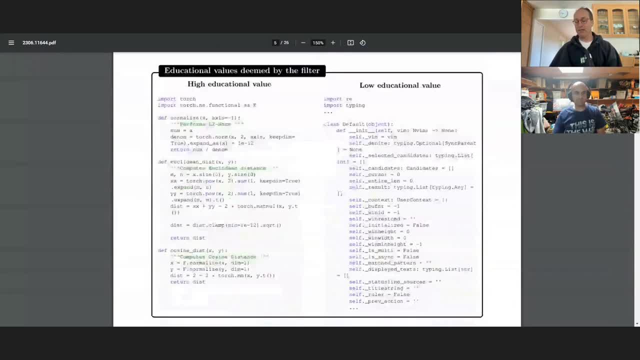 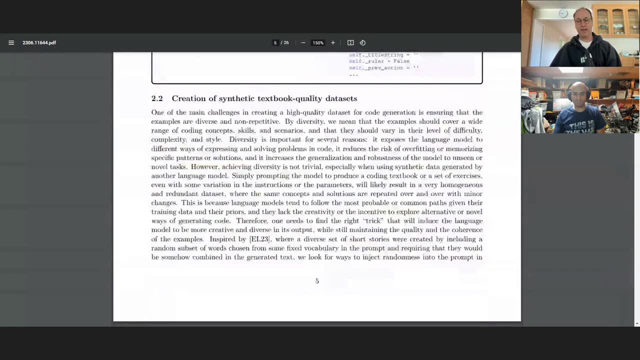 We're cleaning up the quality of that training data. And in a lot of cases, we're generating training data using existing models, and then also using existing models to check the data and see if it's good training data. 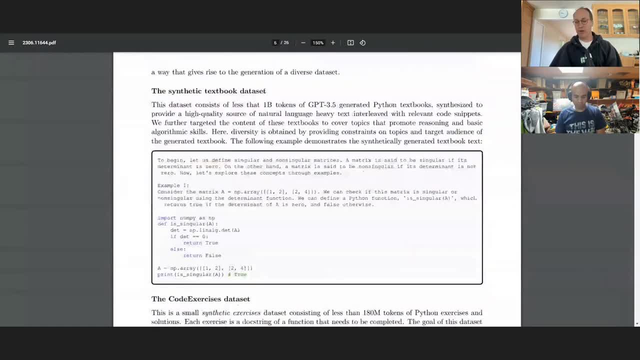 The question I think for us will be, can you go the other direction? That is, use smaller or less mature models to curate training data for a future larger or higher performance model. So far, it's usually been the other direction. 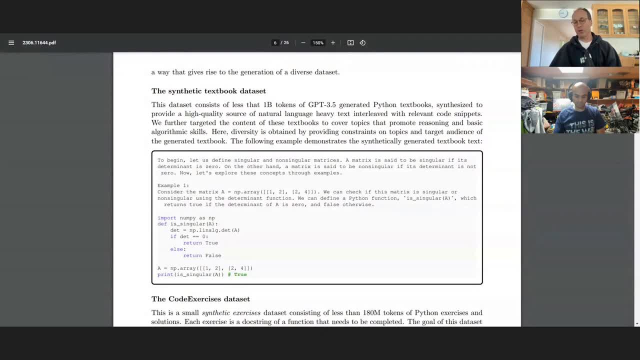 The bigger, really established model is helping you curate training data for a new but smaller model. So these models would serve the same function as human data labelers, but it's, I guess, the next step of them actually creating the training data, 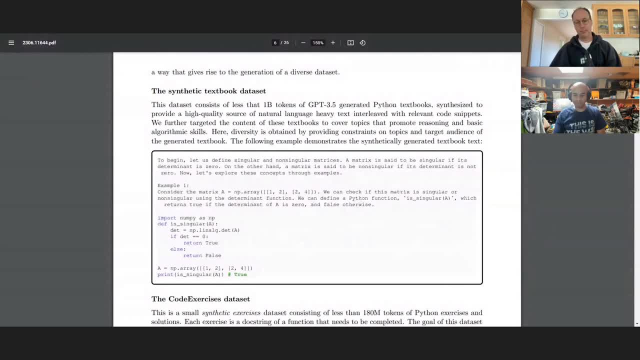 tagging it so that a future foundational model can review it, which should probably save a lot of money. 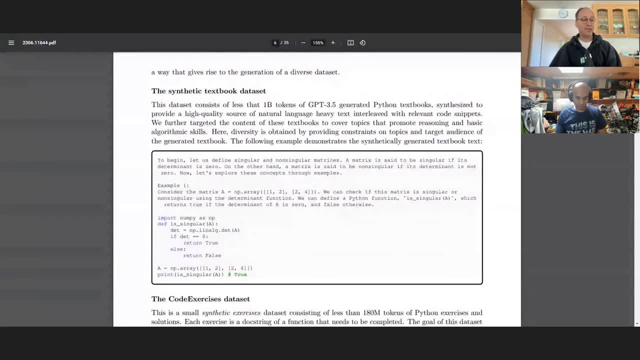 Exactly. Save a lot of money and also get us out of this bottleneck where we're worried that the amount of available training data on the internet is, I should reverse it, we're worried that we've already used all the available data. 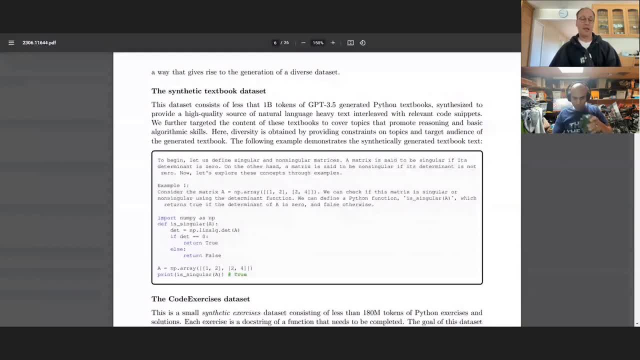 This approach says, no, you can just synthesize the data you need. And furthermore, you can create precisely the kind of data you need for the sort of training that you want to do. So then you probably could create super fine-tuned, smaller models that are not as big as foundational models for specific, like, niche use cases with less parameters and they're cheaper training. You can get it done faster. And they're already demonstrating that in this paper. 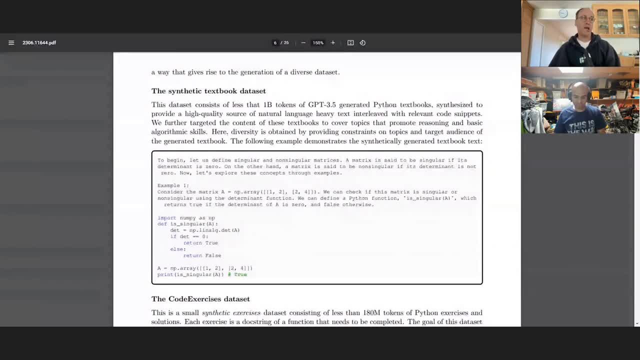 The question I was asking earlier is, can we train equivalent models or potentially even bigger or more powerful future models using synthetic data from the smaller existing models? But yet to be seen. Do you think that's the next logical step? 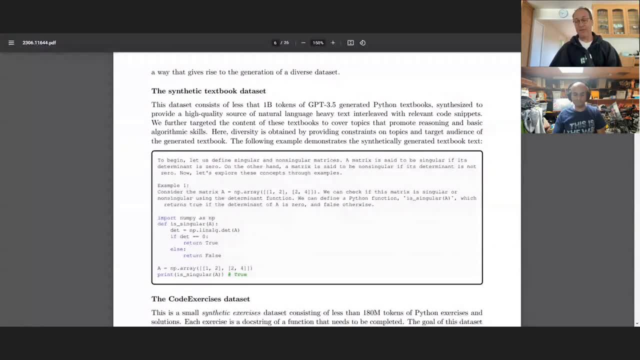 They're going to try to play with that idea? I think so. I think that's the obvious thing to try. Intuitively, it doesn't seem like it would work. Like, how would we train a more powerful model from data generated by? A less powerful one. But maybe you can bootstrap that way. I don't know. 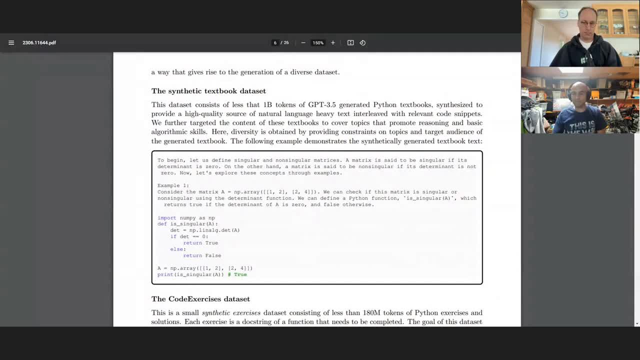 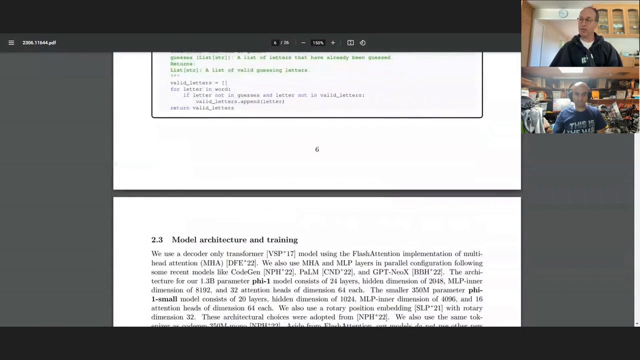 What do you think the implications are for companies that are raising, like, Pi raised a financial round of $1.3 billion to build their own model? Do you think we're going to look back in the next couple of years and be like, actually, they didn't need to spend that much compute or money to get a good model going and they might have wasted their money? Oh, definitely. There's a whole bunch of reasons why you might have wasted your money. One reason is that the training sets and the way you learn could improve your model. Yeah. I think that's just guaranteed. 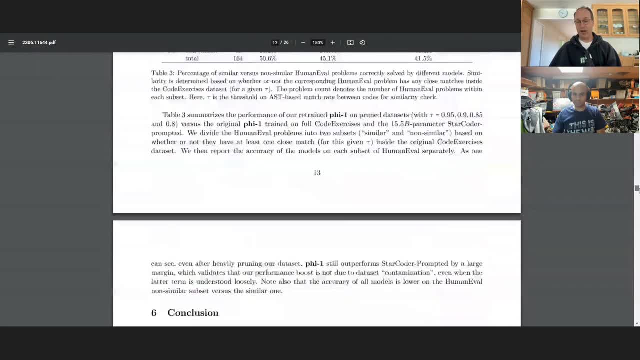 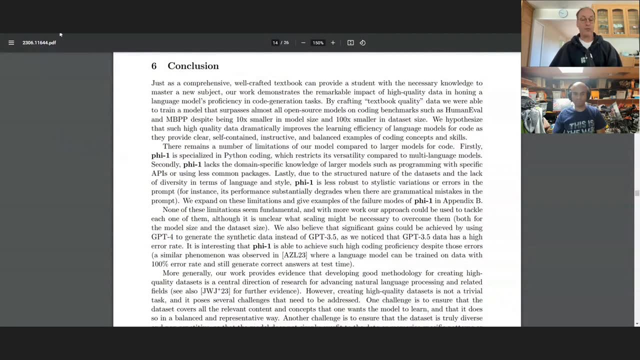 There's so much research happening in so many areas to improve the training and to improve the training set. I think it's given that we're going to get much better at it, but that applies to everyone, right? 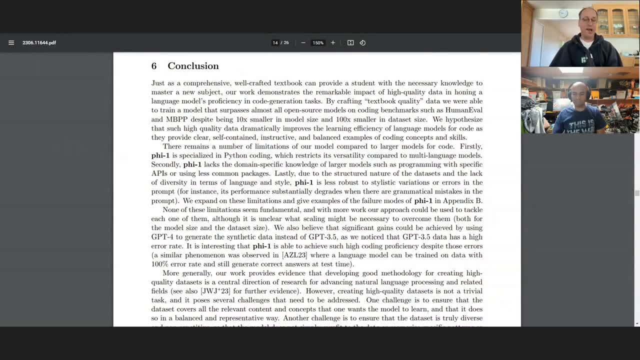 Everyone's going to look back and say, oh, my God, we used to train models this old way. It was super expensive and super painful. And now we're smarter about it and we can train a better, faster, smaller model with less effort, blah, blah, blah. 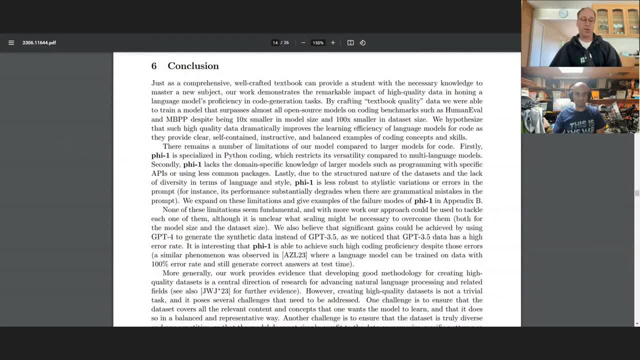 I think that we'll see that a lot of funding went into it. I think that we'll see that a lot of funding went into it. I think that we'll see that a lot of funding went into a lot of models that probably was overdone, but also that just the sheer number of foundation models might be overdone. 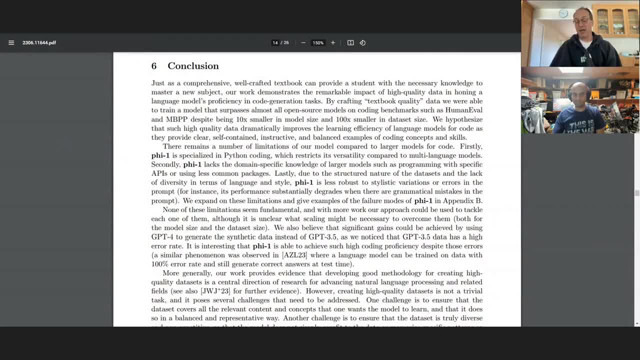 Do we need more than three large foundation models? I don't know. 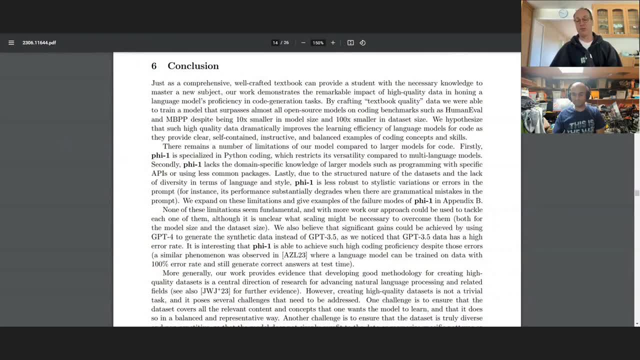 I'm not sure what to do with that many. I think that more special purpose ones are more interesting at this point. 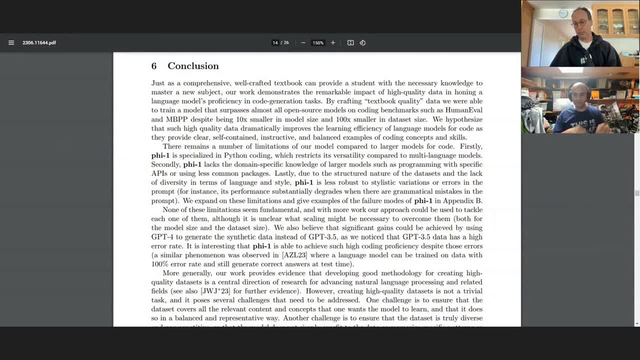 That's true. Some more special purpose ones focusing on health care or scientific research and discovery or maybe like a legal foundational model. 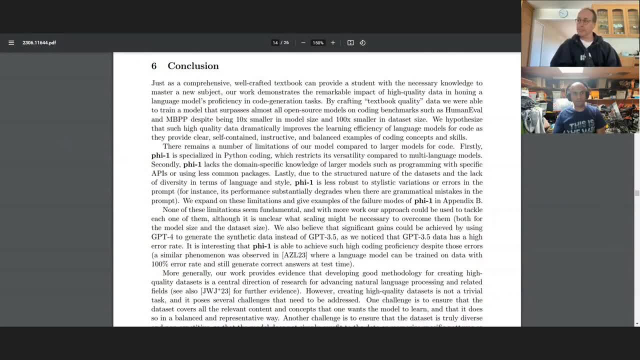 Yeah. And I think we might see right now we're seeing a range. It's a great place to see who can get the best foundational model out there. 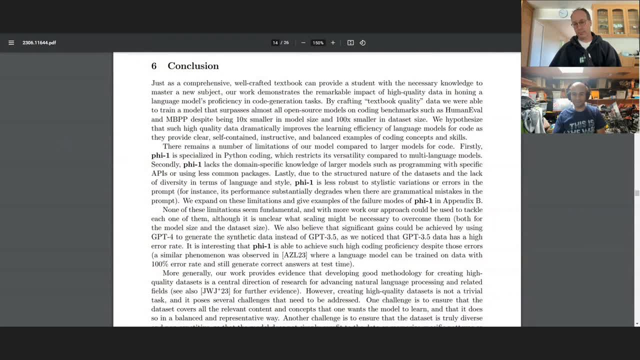 But there's eventually there's going to be consolidation probably on the user side saying, hey, actually, I'm good with open AI. Maybe Pi and bar are good enough. 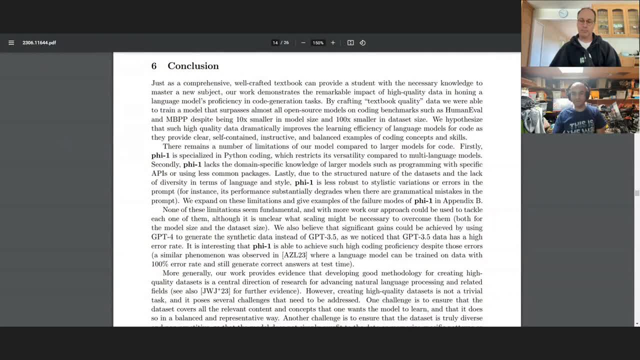 And as far as like these 50 other foundational models, maybe people aren't familiar enough with them and aren't willing to try this service. So they're more willing to say, no, I'm going to stay with the top three and go from there. Maybe it's similar to what we see in the cloud space. Yes, there's Amazon. There's Google. There's Microsoft. There's also these other small providers. People haven't really heard of, but mostly when people are thinking about putting their applications on the cloud, they think the big three and the rest are just not even thought of. I think that's a good summary. 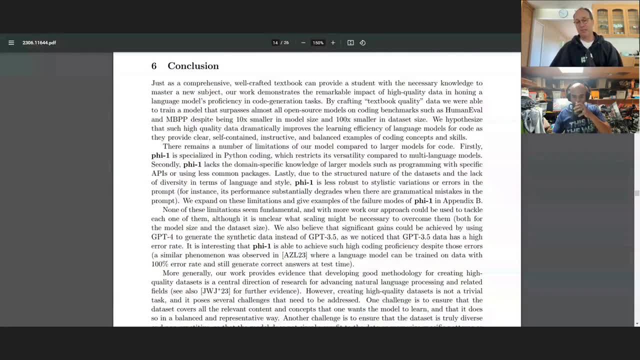 I'm not even sure it's big three. I don't know how good the analogy is, but if you go back and look at search engines, there was a time where we had, I don't know, 10 or 12 big search engines and they were racing to see who would get the most market share and who could handle the largest collection of documents and who had the best relevance and so on. And honestly, it's. That's the world's most popular. The big three. And it was easy for us to understand that you could use web crawler to find all of these things. 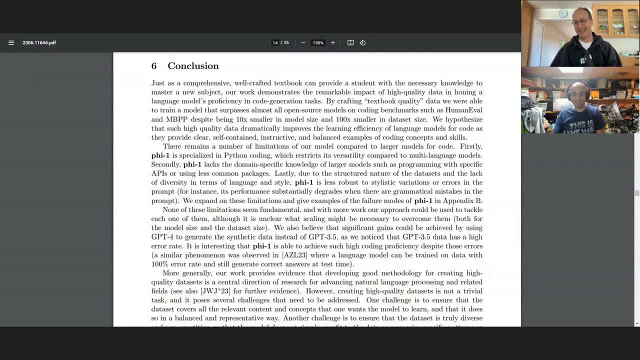 You know, we're not into the digital industry anymore, but I would say it's easy to find these things, but if you think about the numbers and you're not interested in them and they're not, they're not going to solve those problems for you. But once you did Google and Google found one of these, you know, thousands of... That's the cloud service and you think, I don't know, this isn't like the... You know, you can't use the Google software and you can't find something like that. You know, you can't use the cloud service and you can't find something that doesn't really fit your needs, which is... 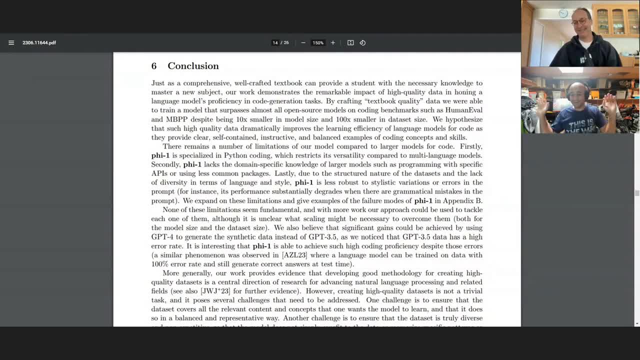 for free yes i'm on google and then 10 years later i work there wow okay joe any last thoughts on this paper anything that you think there's really anything that caught your mind before we move on 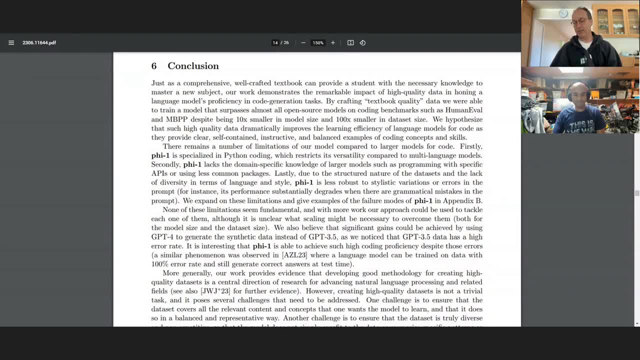 to our next topic i think this idea of producing synthetic data sets will still have lots of follow-on research and likewise even though they just started to do it here changing how the model 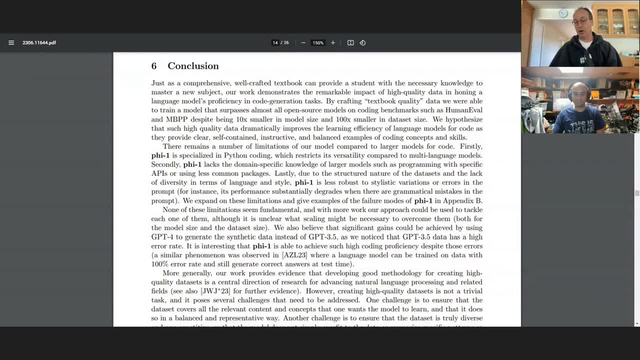 is trained will also potentially yield large improvements like we're just doing so much work for the kind of learning we're getting and we have an existence proof in organic systems that's us 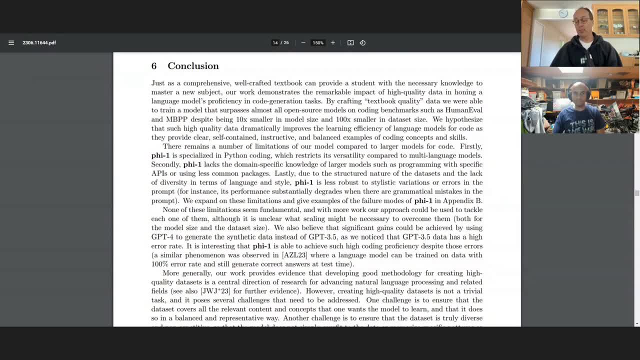 and maybe some primates that learning could be much faster with a much smaller set of examples